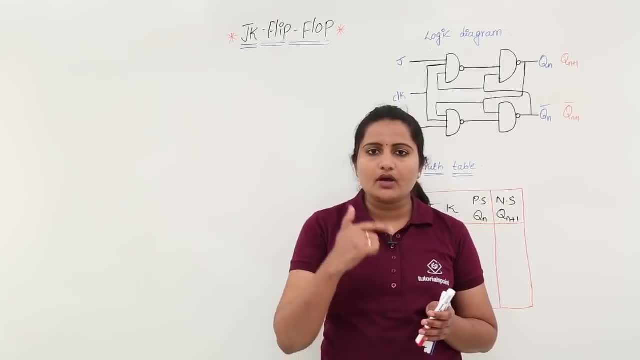 If you take an SR flip-flops with set and reset, you have a no change condition. but if you take an SR flip-flop, one condition is going to waste. one cycle, one time cycle for S equal to SR equal to 1, 1 cycle is going to waste. So that is why we are going to discuss about SR flip-flop. 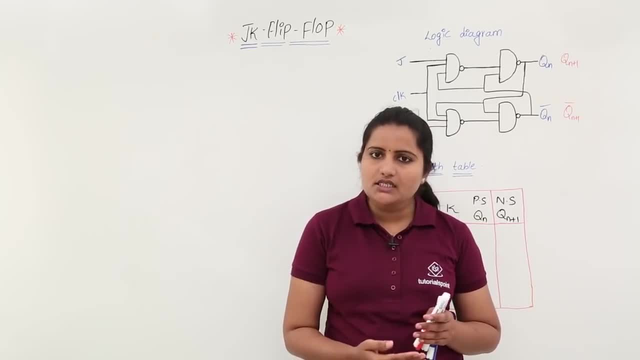 So in that case, to change that indeterminate state, to use that indeterminate state, we are having another circuit, So that indeterminate state we are changing, like toggle state in that particular condition of SR, is equal into 1, 1.. So that state, that circuit will provide 1, 1.. 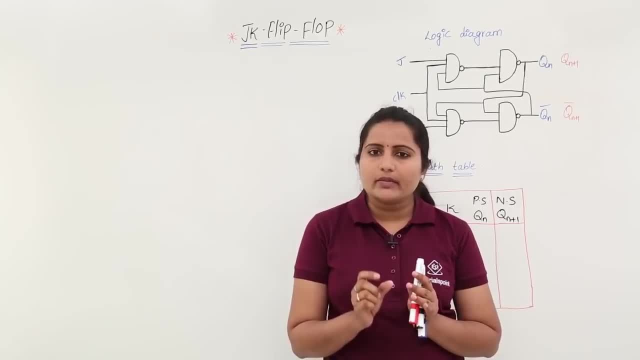 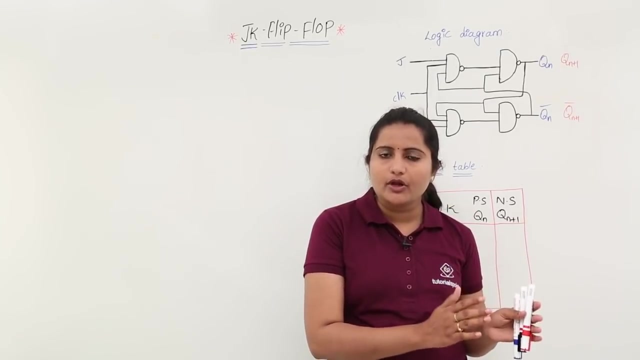 So same for same SR flip-flop. we are making a small change to work as JK flip-flop. The main use of that JK flip-flop is we are toggling the inputs. That means whatever indeterminate condition in SR flip-flop, indeterminate state: is there that state we are using here? 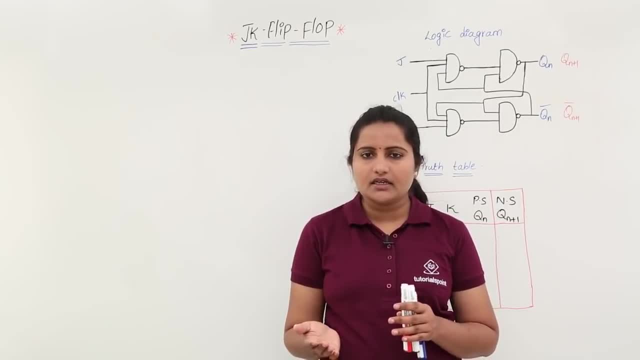 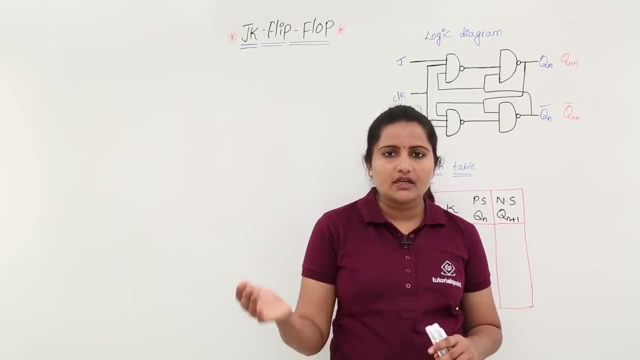 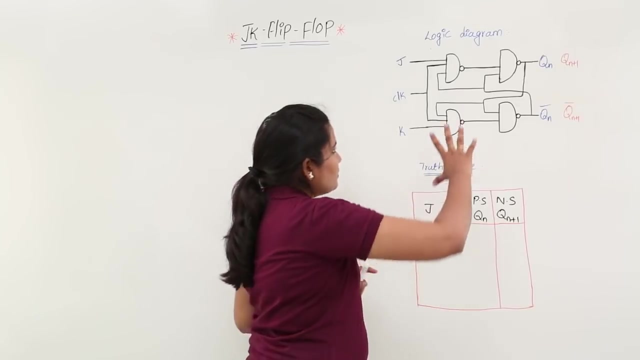 and we are. we are changing that indeterminate state to toggle state. That means whatever SR is there, the toggle of that SR will come. That means here we are naming that SR as JK. So now just you know that this is structure for SR flip-flop. the only change we make it. 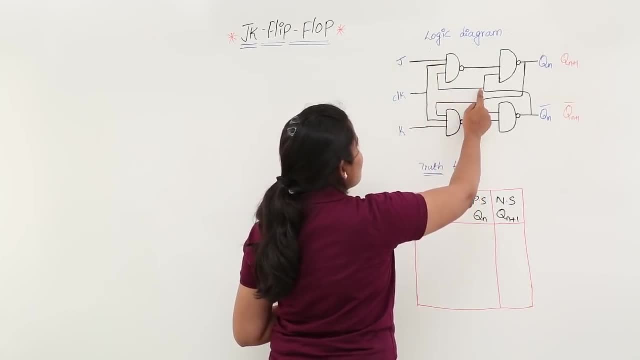 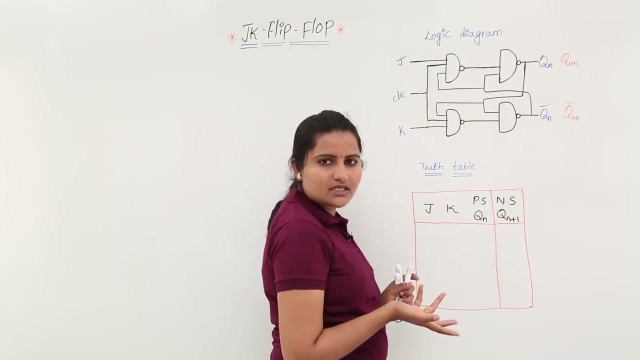 for this to become like JK flip-flop is we change it like this. So we given this connection here, also previously in SR flip-flop. we are not having these two connections. Without these two connections and inputs are as S and R. this this is nothing but a SR flip-flop. 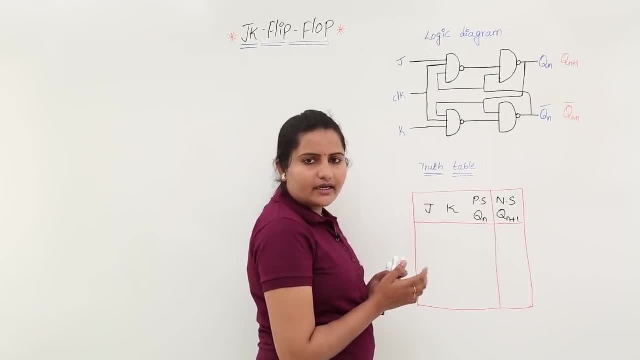 So to make use of that indeterminate condition, we are designing this JK flip-flop. So in that indeterminate condition we will get toggle state now. So here we will see. we we taken just this feedback to this previous gates also, So now I am propagating the inputs. 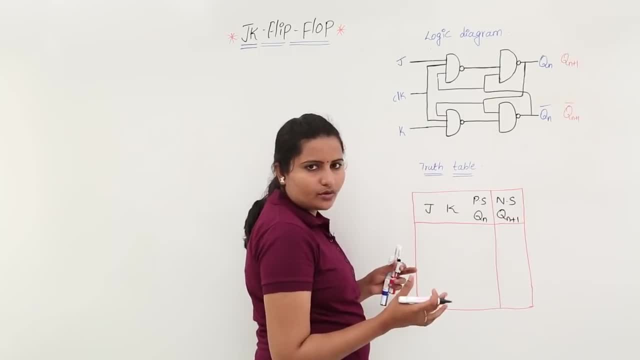 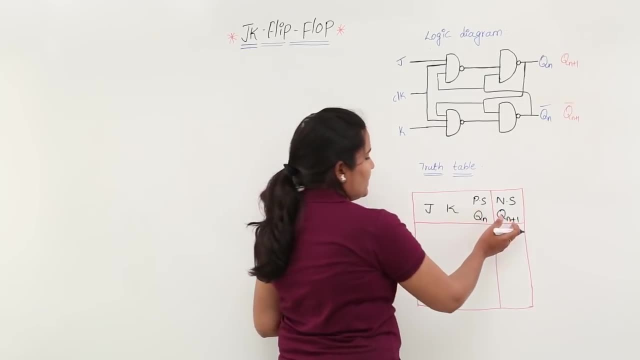 So, as usual, your present state. you do not know The. the required output for any sequential circuit is your next state only. So next state means Q n plus 1. So this you need to determine. So here you do not. 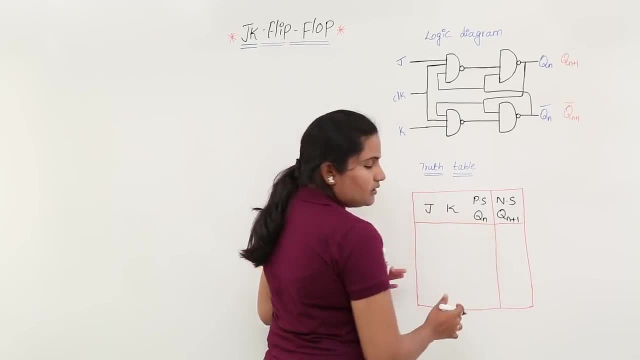 know your present state. So that is why you can take do not care at the present state value. So here your JK inputs may be anything like 0, 0, 0, 1 and 1, 0 and 1, 1.. So you do not. 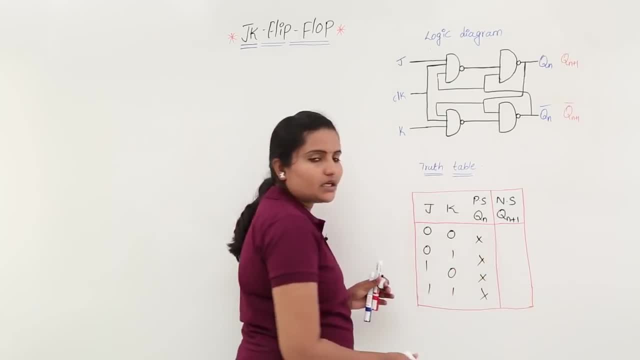 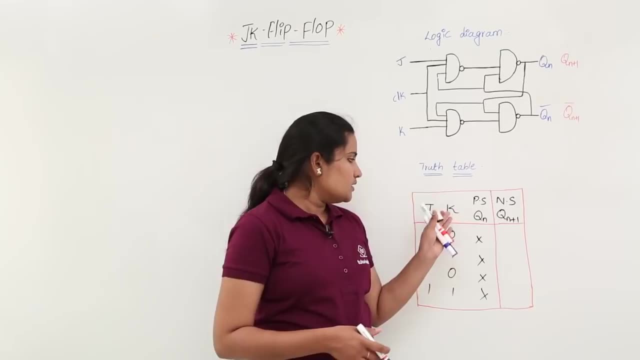 know your present state at any value. So that is why I am just taking- do not care- the present state. So you need to take either 0 or 1 for that do not care present state, you need to take next state. So now I am taking this first condition, So I am just taking this first. 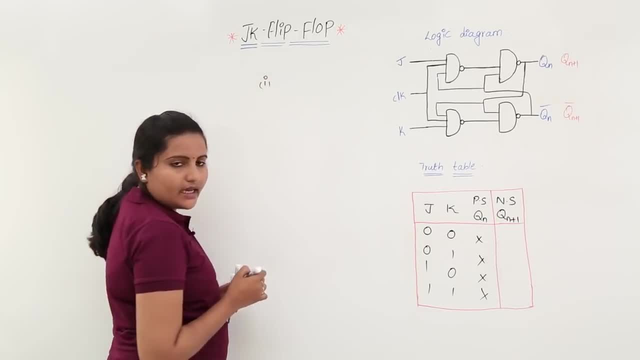 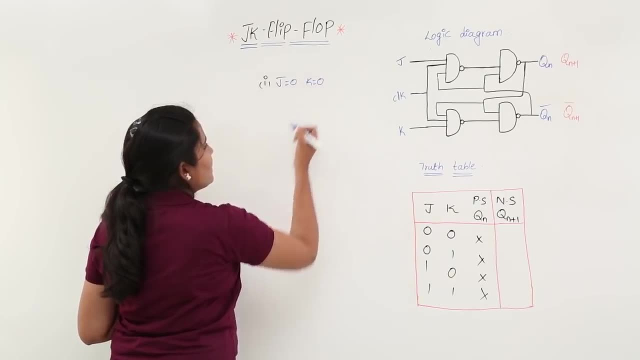 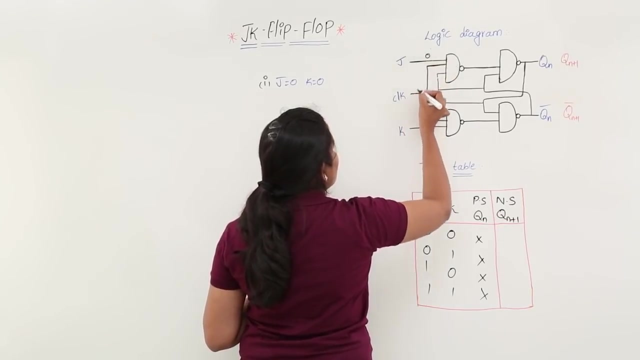 condition: J is equal to ah, k equal to 0, J equal to 0 and k is equal to 0.. This condition- I am considering- always clock must be- is equivalent to 1 here. So here I am just considering J equal to 0 and k equal to 0.. 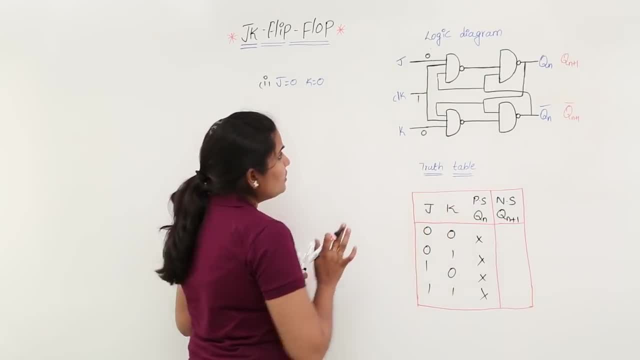 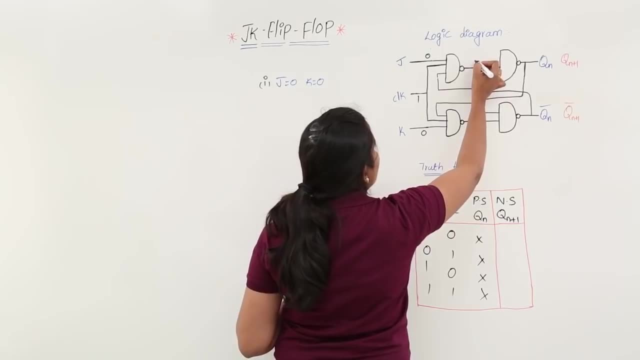 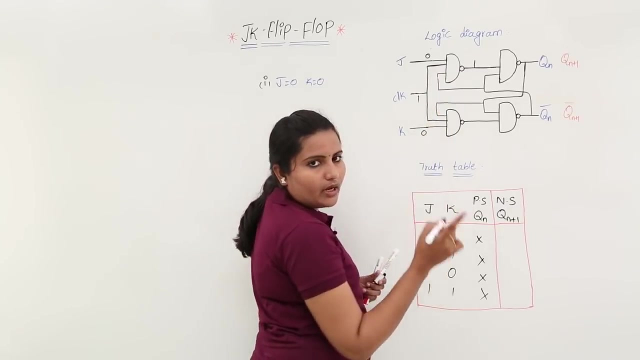 Now see here: 0 into anything other. 2 inputs is equivalent to So 1 here. So 0 into 1 whole bar. you are getting 1 here. So 0 into anything whole bar. you will get 1 here Now. 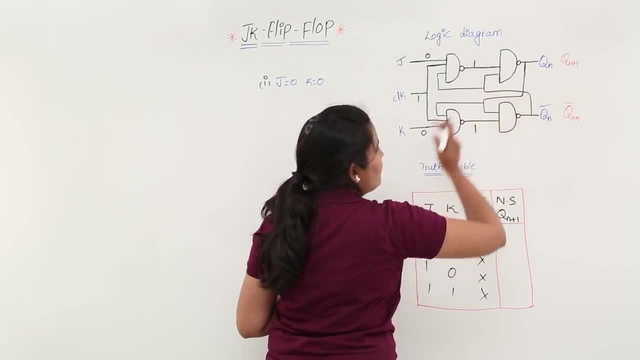 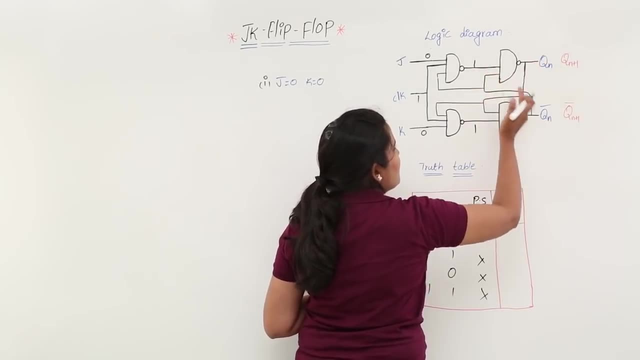 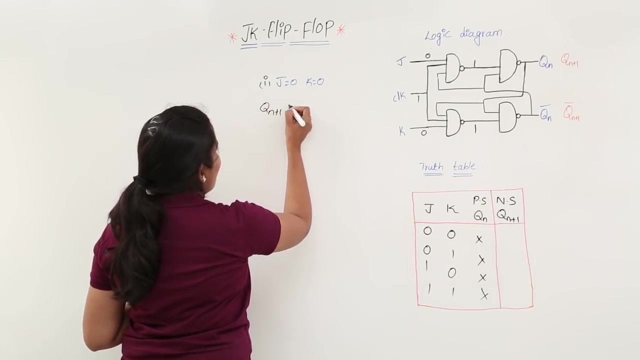 you are crossing this one with this Q n bar. So what you are getting at Q n plus 1 after crossing these present states, what you are getting is Q n plus 1 only. So here you are: Q n plus 1. that means your output is equivalent to. so 1 into your Q n bar, whole bar I am. 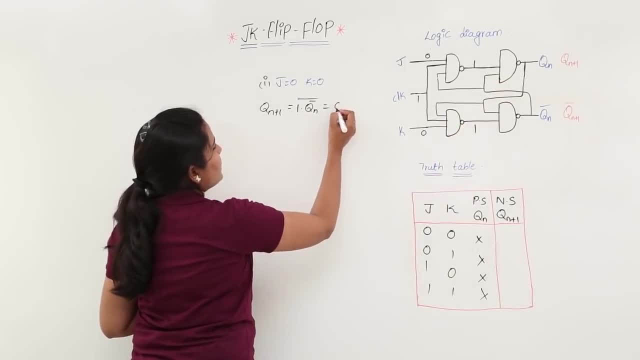 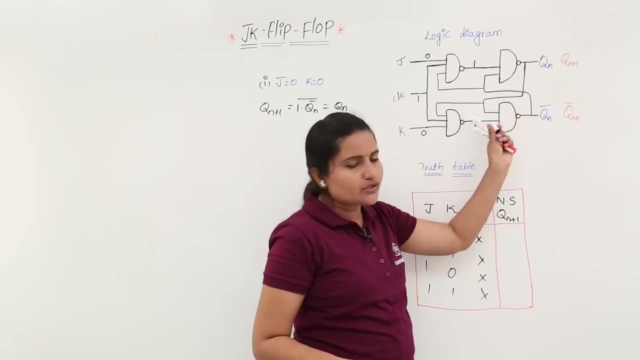 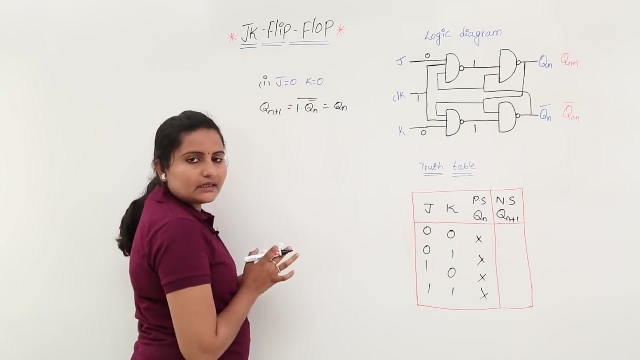 just crossing this gate. So now this is equivalent to Q n. whatever already is there. you got same thing by processing these inputs to inside. So that is Q n plus 1 is equivalent to Q n. So you do not know this q n value. that is why, to guess this q n value I am going for 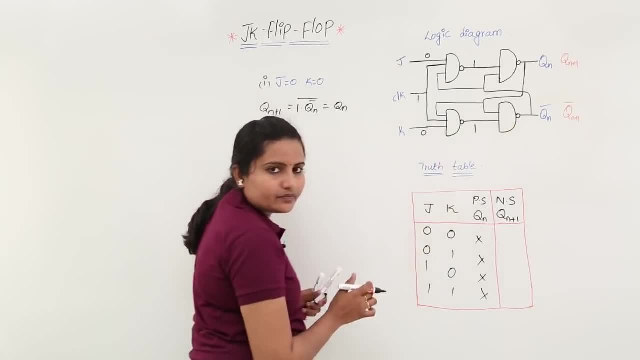 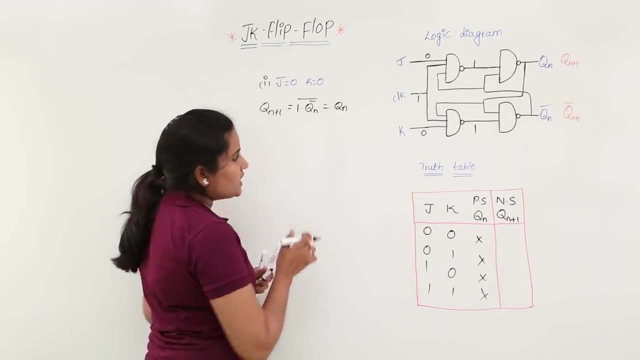 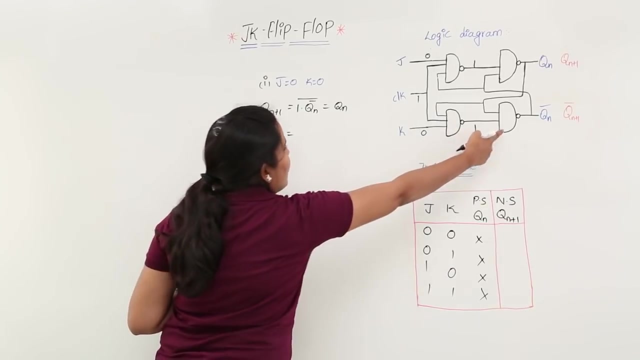 complement port. that means I am processing this gate. If you got any value here, no need to go for complement port. here you go. you did not got any value up to now, So that is why I am going for complement port. that is q? n plus 1 bar. This is equivalent to: I am just processing this gate. 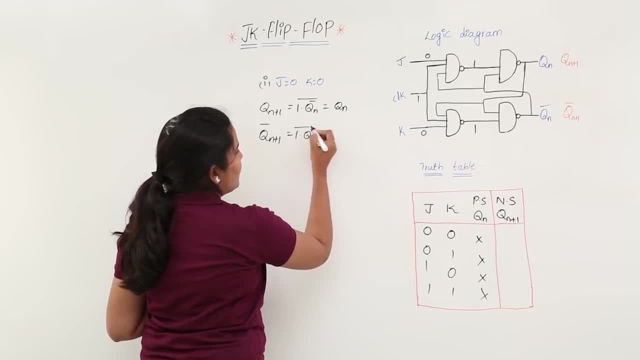 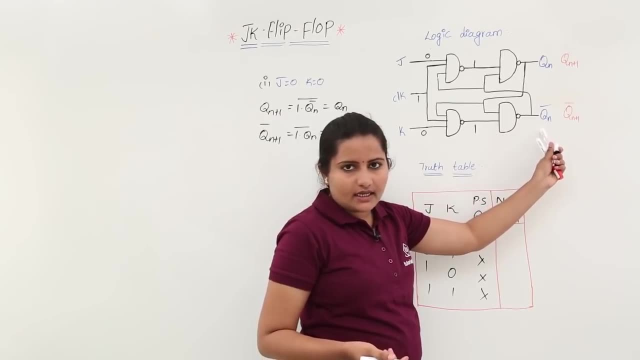 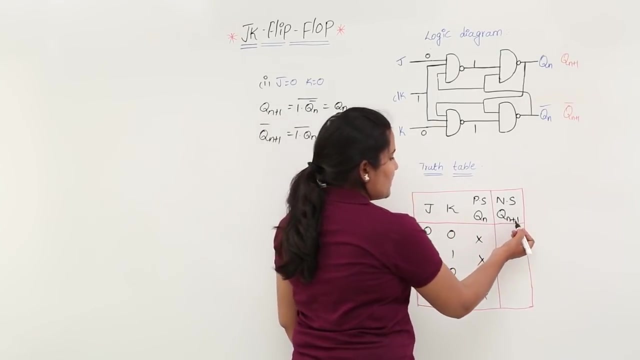 So 1 into q n whole bar, you are getting q n bar. So you can observe: whatever present state, outputs are there same you got like for next state also. that means no change. So whatever q n plus 1, q n is there same, coming in the place of q n plus 1. you can observe here: 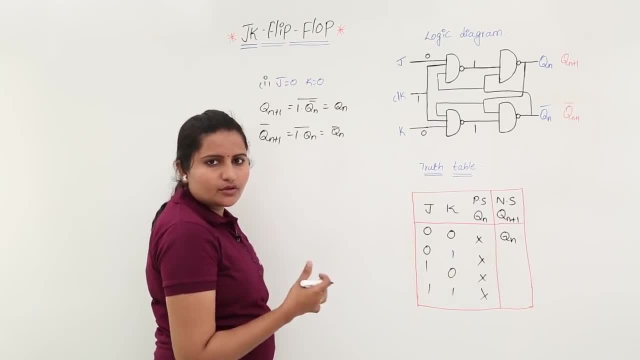 Why we derived this means to observe, to check whether we are getting any Q n or Q n plus 1.. So you can observe here. So you can observe here, So you can observe value in complement port or not, When you are not getting value. here that means 0 or 1, you need to. 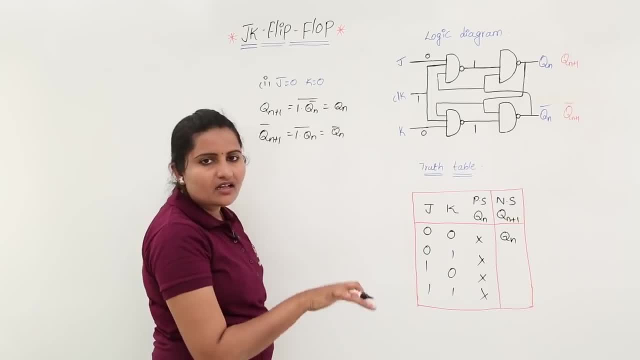 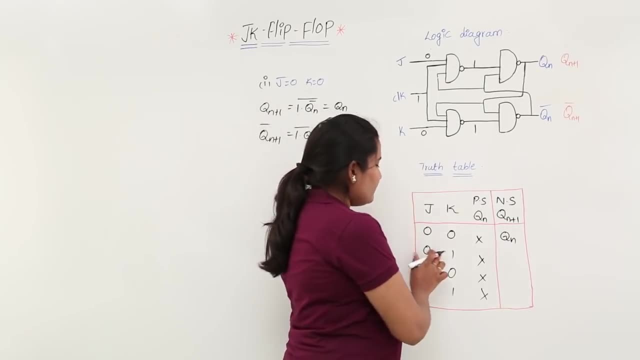 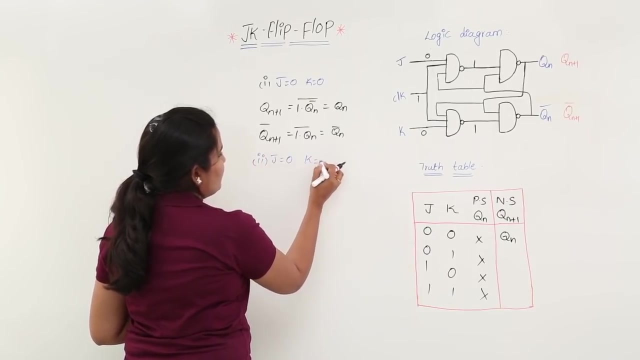 check for complement port for value. Even here also, you are not getting means. you can write as it is. whatever you got, then you can write as it is. So now I am going for this condition. the second condition is equivalent to j, equivalent to 0, k, equivalent to 1.. So j 0 k is equivalent. 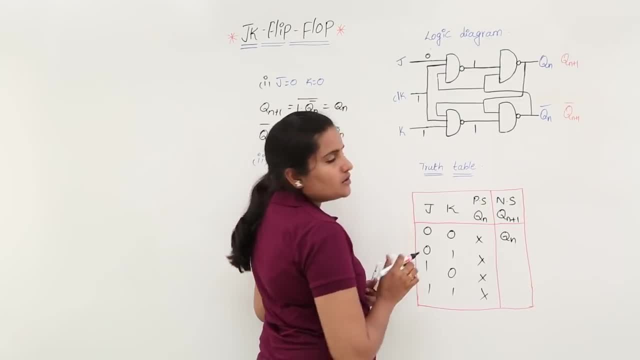 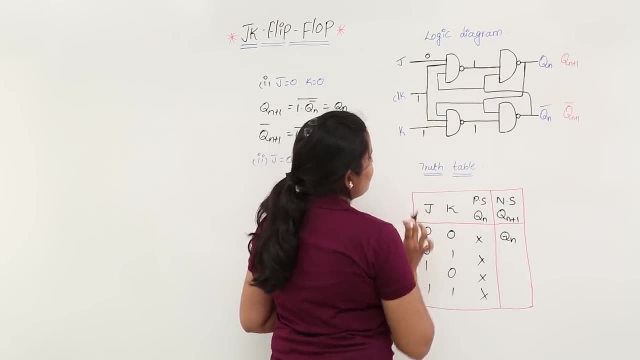 to 1.. Now see here. So 0 into anything is whole bar is equivalent to 1.. Now see here. So here you are having 1 into clock, another one into, So where you are taking this input. this input is coming from q n, So here your. 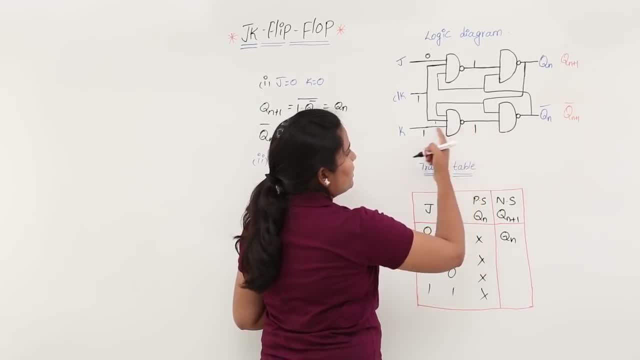 output may be So: from this gate, output 1 into 1 into q n. So from this gate, output 1 into 1 into 1 into q n. So here your output may be n whole bar. you are getting q n bar here. you are getting q n bar here. So now I am just 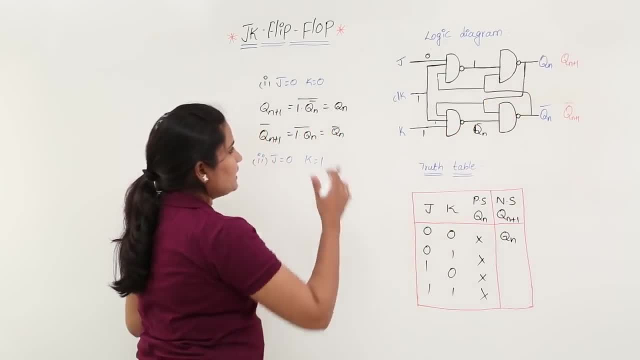 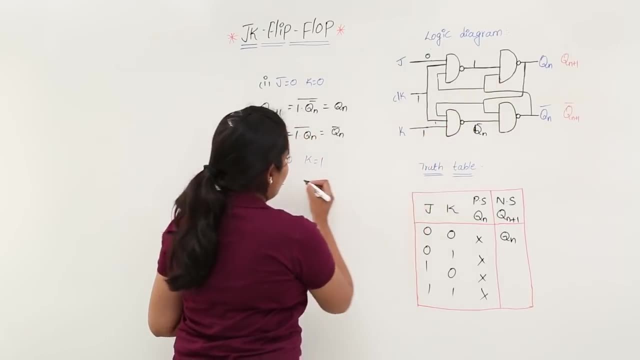 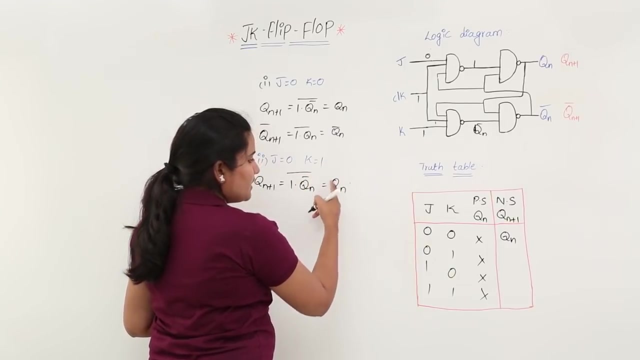 propagating this gate. I am just propagating this gate, So top gate. I am propagating q n plus 1 is equivalent to, So this gate. I am propagating 1 into, So q n bar, whole bar. you are getting q n here. I did not got any value here. to check whether there is value. 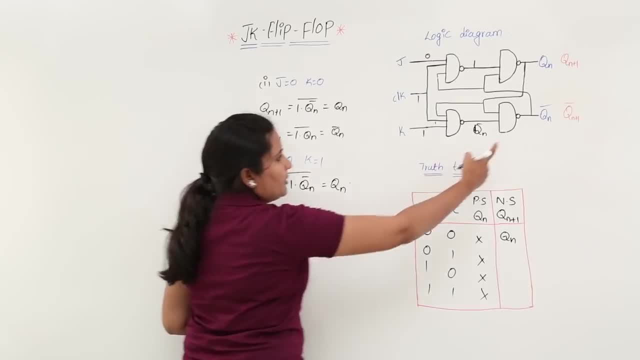 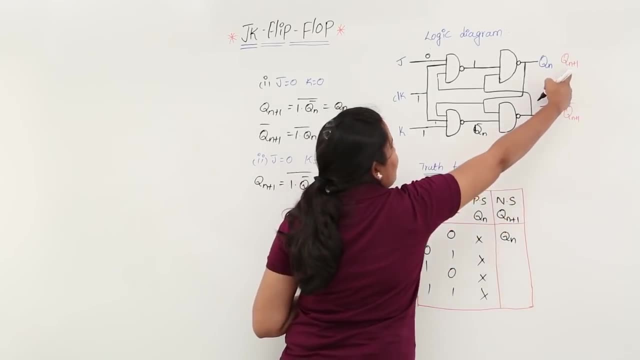 at the complement port. I am going for this gate. So complement port is nothing but this port. So when q n is there, it will provide q n bar complement. So when next state output is there, it will provide complement of next state. like that: q n, q n plus 2 is there it. 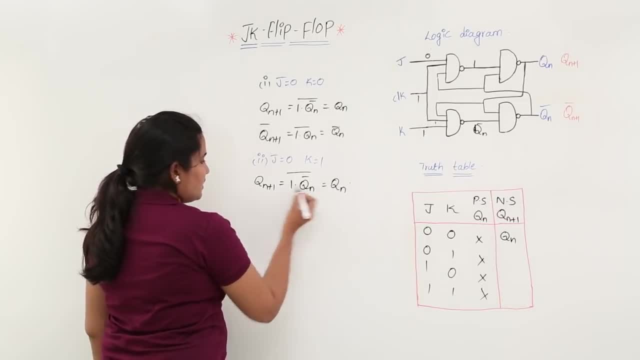 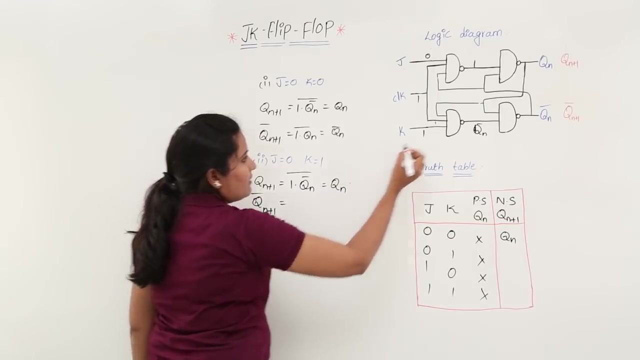 will provide q n plus 2 bar like that. So here to check whether we are getting any value in complement port. So I am checking this q n plus 1 bar, So to get q n plus 1 bar. I am just propagating that q n to q n bar. So I am, I am having q n bar here and q n. 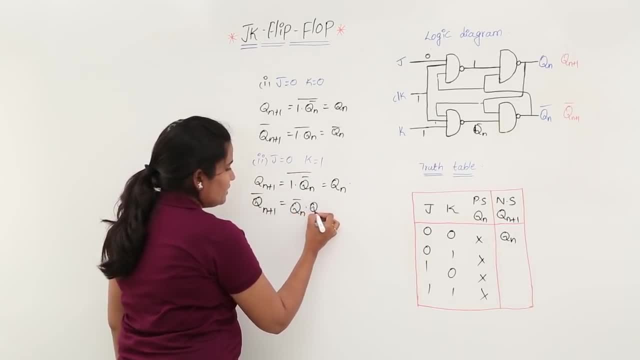 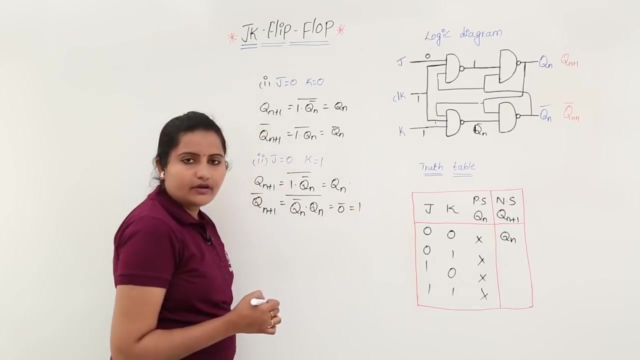 here q n bar into q n whole bar, So a into a bar equal to 0, 1 into 1 bar equal to 0, like that. anything and its complement, if multiplied, will provide 0. So 0 bar. it will. it will. 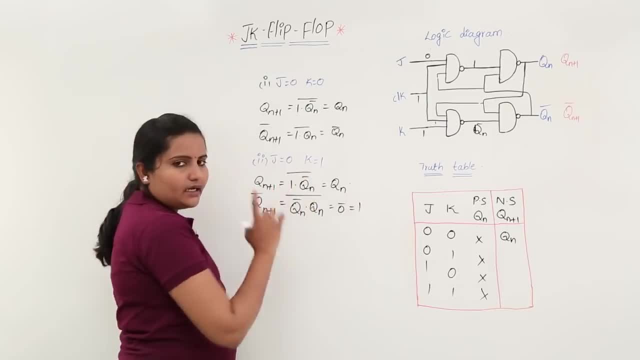 give you 1.. So here you are getting your q n to q n bar. So this is just propagating the q n power to 0.. So it is just propagating the q n to q n bar and just propagating the. 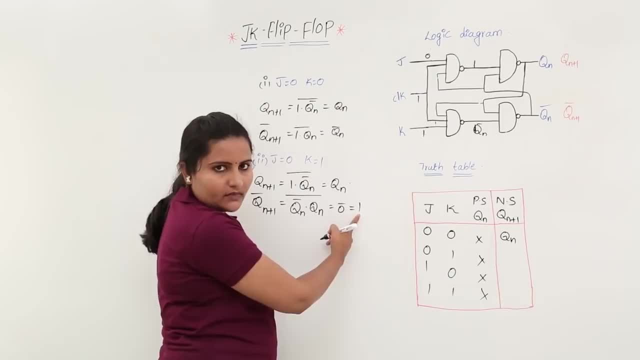 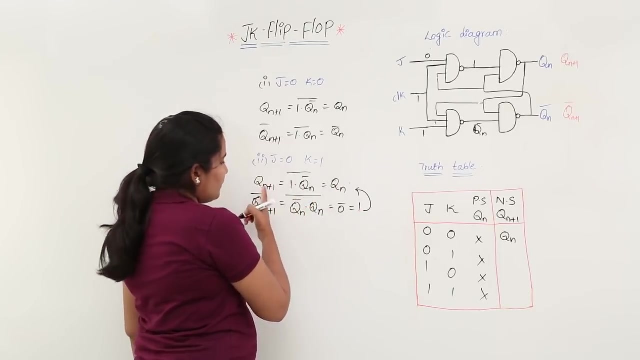 q n plus 1 bar is equivalent to 1.. Yes, you got value in complement port. This you can use as reference to get value at normal port. If q n plus 1 bar equivalent to 1, you can implies that your q n plus 1 equal to 0. That means your q n is equivalent to 0. This you can put 0. This is. 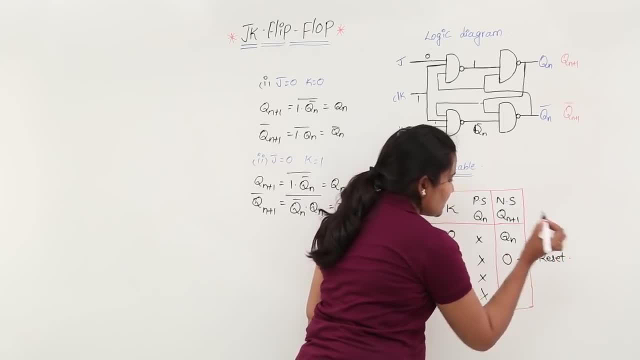 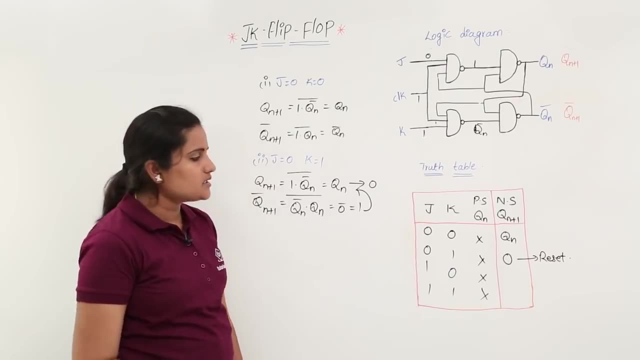 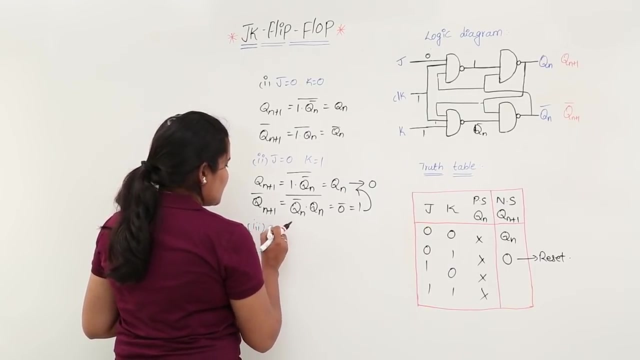 called as reset condition of your j k flip flop. When j k flip flop is going to reset means when j equal to 0, k is equivalent to 1, that is called as reset. So now I am taking my third condition. Third condition is: j is equivalent to 1,. 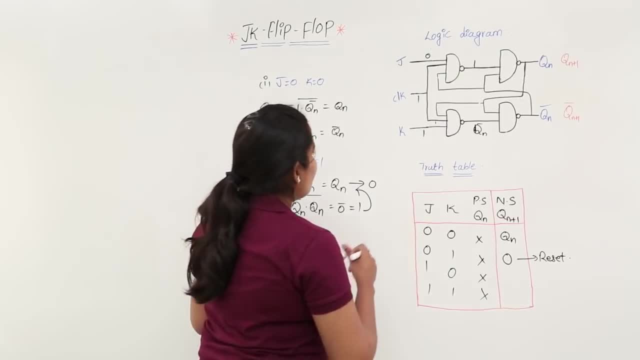 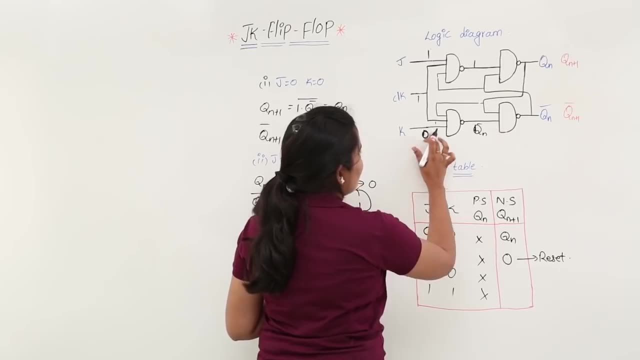 k is equivalent to 0. So now I am taking: j is equivalent to 1 here and k is equivalent to 0 here. If k is equal to 0, without knowing two inputs, this gate will provide 1.. And top side, if you can see 1 into 1, into this is: 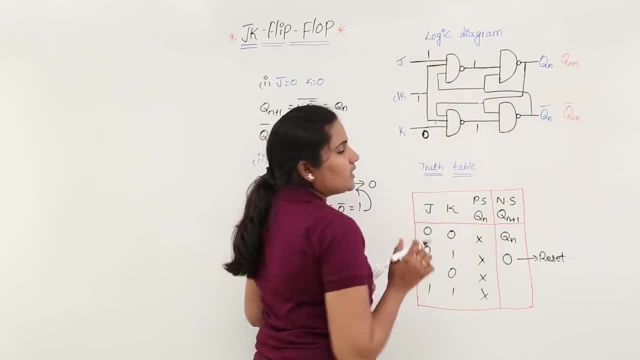 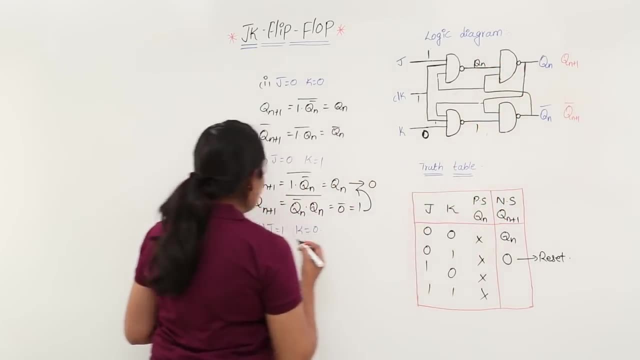 coming from q n bar. you can observe here 1 into 1, into q n bar, whole bar. you are getting q n here. So if you observe this, q n plus 1, if you are writing for q n plus 1.. So this is equal to. 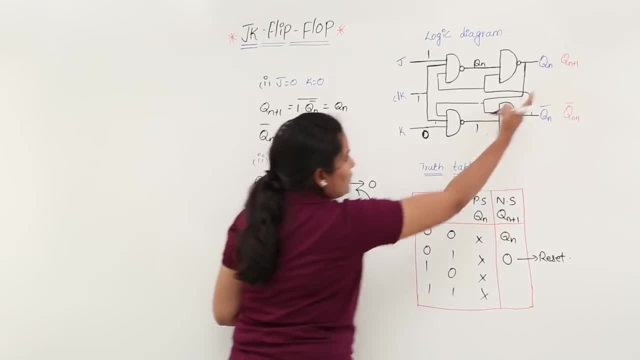 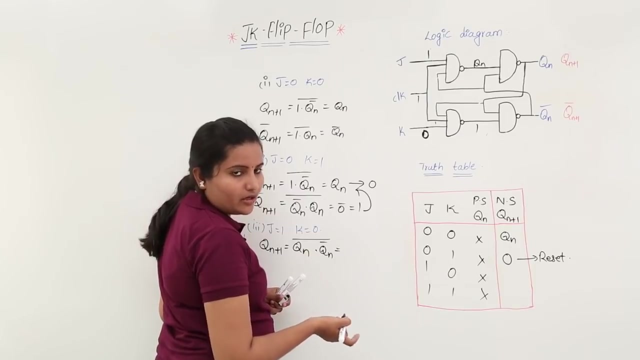 so q n into. to get q n plus 1 you need to process this present inputs, So q n into. downside you are getting q n bar, q n bar, whole bar. So a into a bar. whole bar means like 0 bar. 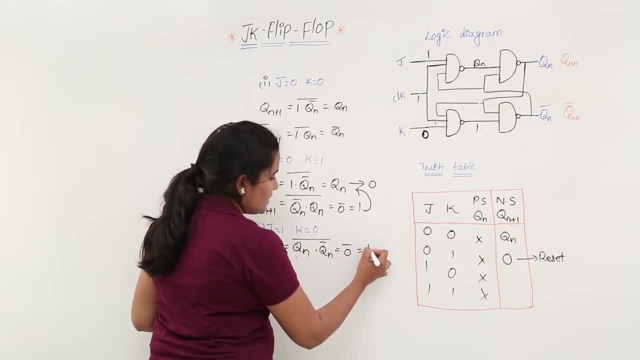 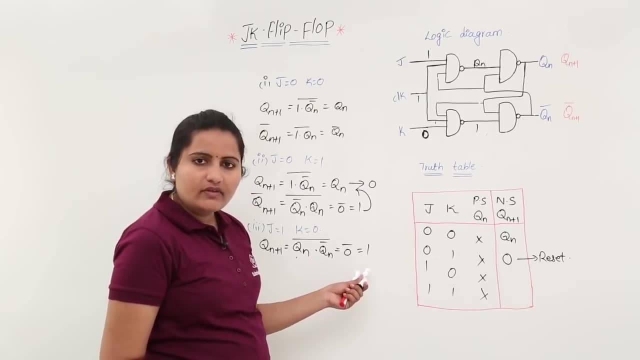 only So. this is q n into q n. bar is 0, bar is equivalent to 1. you already got value. So at q n plus 1, no need to go for complement port now, because whatever the next state is there, you got here only So to, for example, if you want to take your complement of next state. 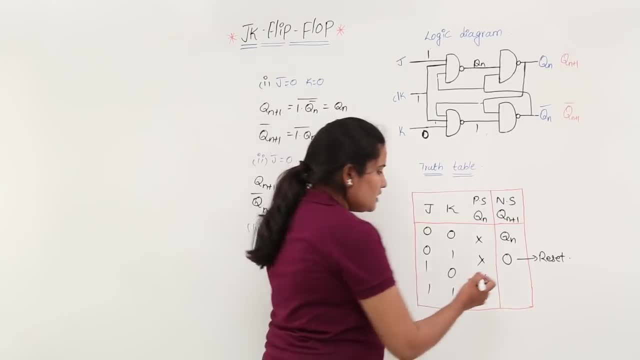 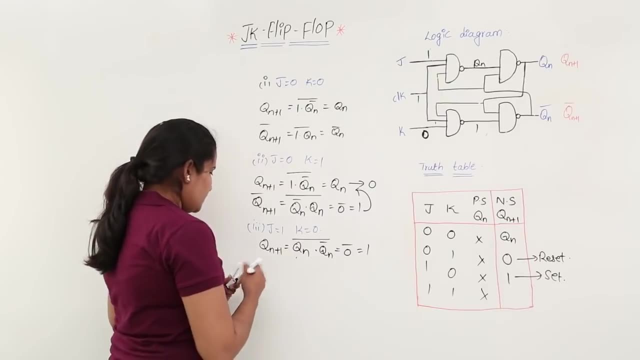 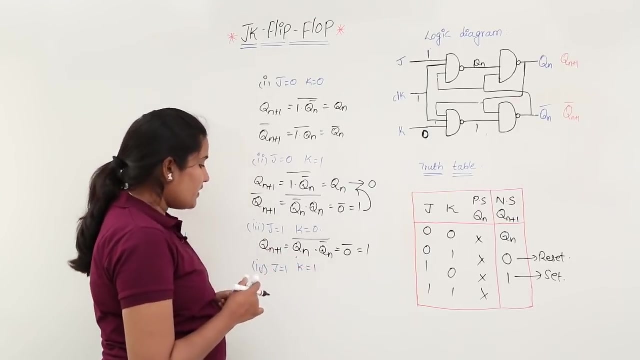 then you are getting 0. only no need to calculate here. So you got in first step itself. So this is called as set condition. So now you are taking your fourth one. this is called as j equal to 1, k is equal to 1 condition. when j equal to 1 and k equal to 1, what you are getting? 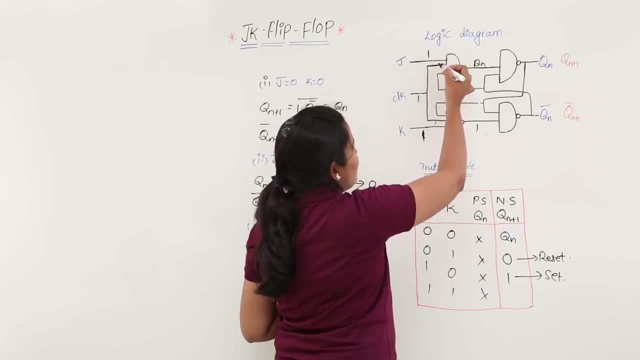 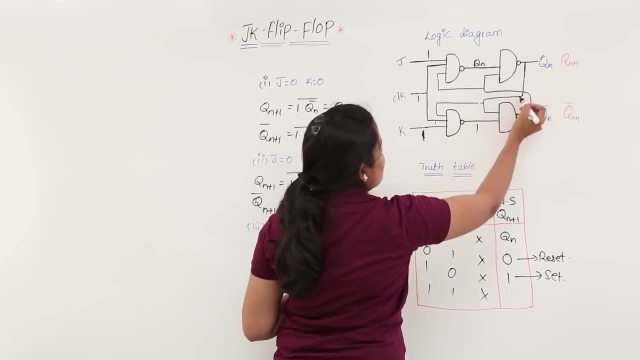 is So when j equal to 1, k equal to 1, 1 into 1 into here q n bar is there, here you are getting q n and here 1 into 1 into this q n will come 1 into 1 into q n, whole bar you are getting. 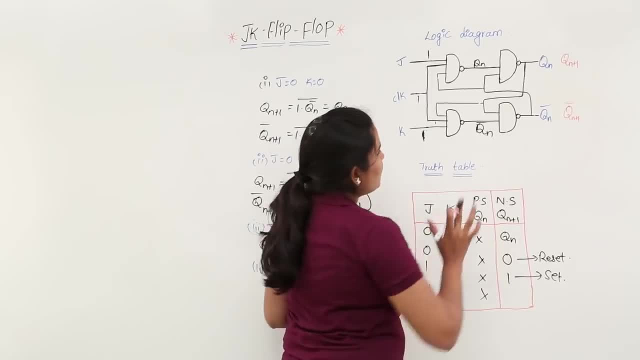 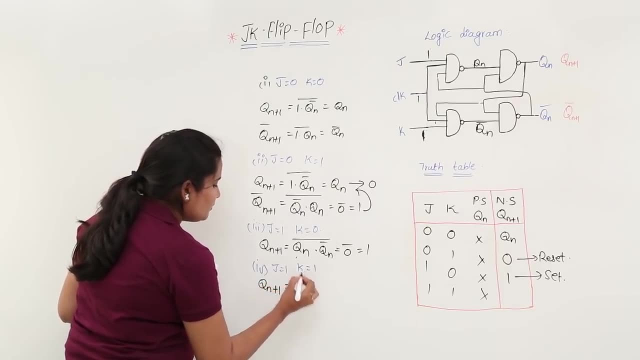 q n bar here. Now see here. so I am just writing like this. so I am writing equation for q n plus 1.. So q n plus 1 is equivalent to. so here, if you want q n plus 1, you need to process this gate. 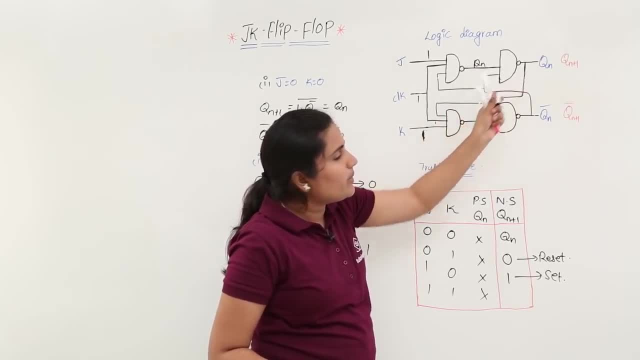 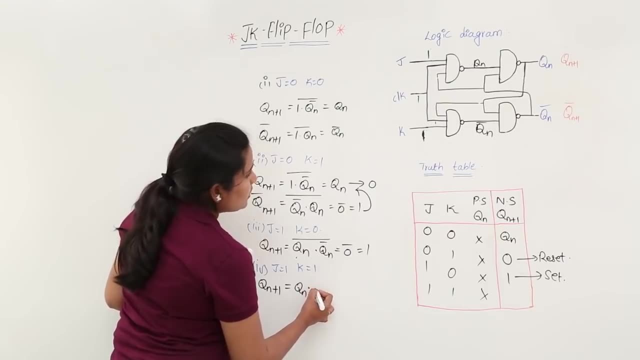 the gate inputs are q n and q n bar. So now I am taking q n into q n bar- whole bar. So that is meant by so here. q n into q n bar- whole bar, means. so here you are getting some 0 whole. 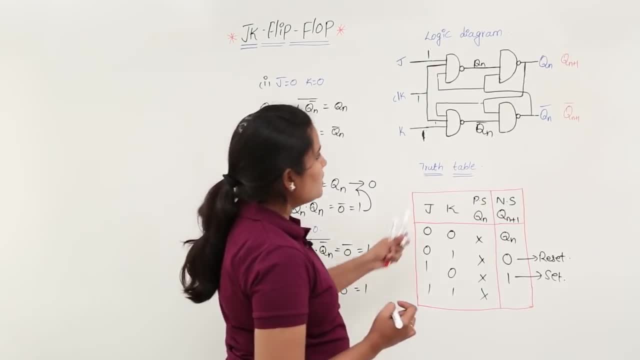 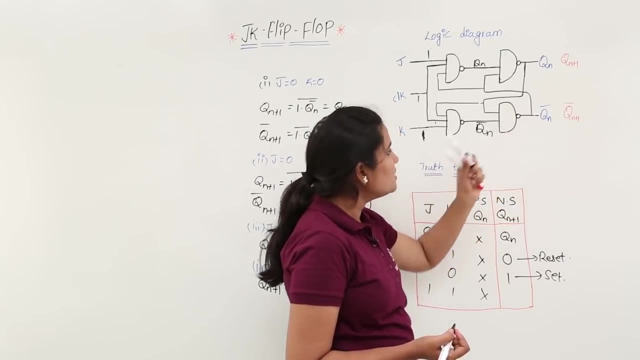 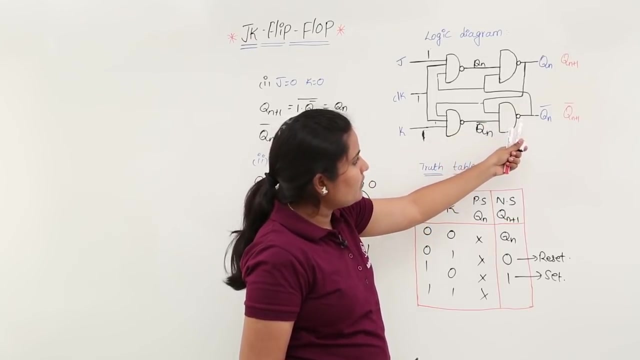 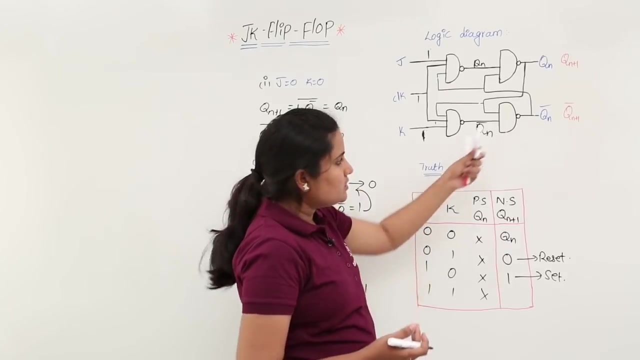 bar. you are getting So now here, if you process at this gate, if you process at this gate, what you are getting, you just check here. So if you process at this gate, so again q n into q n bar will come, So again you are getting same thing. that means, so you are getting so here also 0 bar. 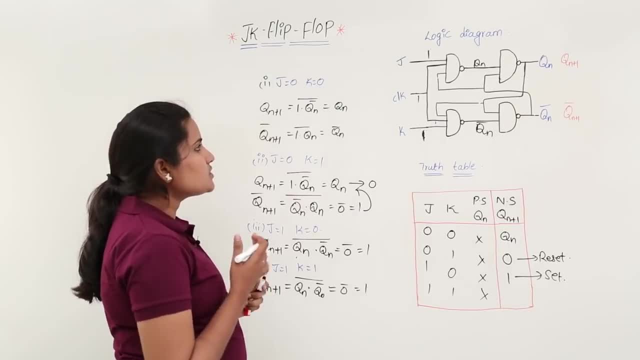 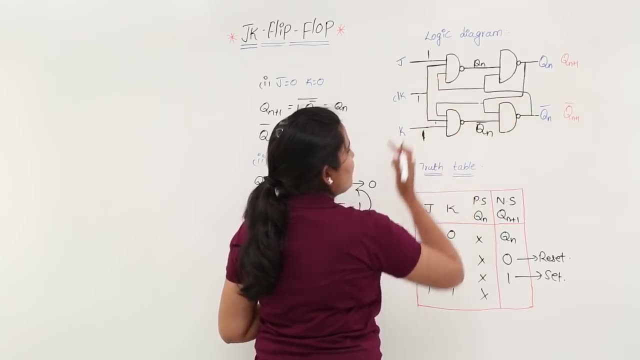 will come. that means 1 will come. So how it will goes to toggle condition means you can check here. So 1 into 1 into when you taken this q n bar, you are getting q n and here 1 into 1 into q n. here you got q n bar. Now I am just deriving the output of